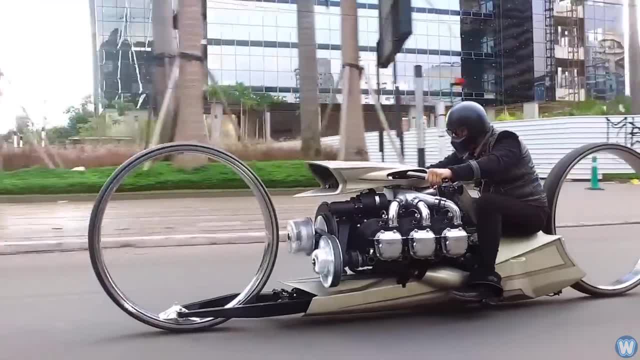 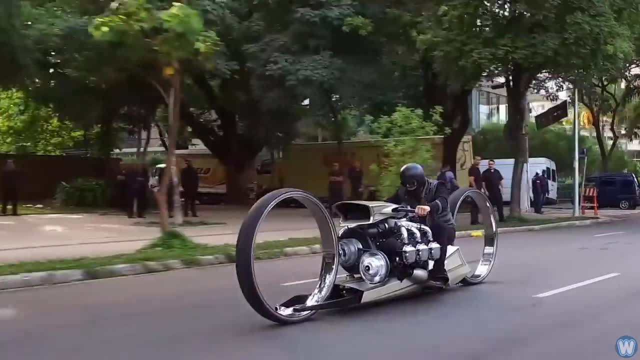 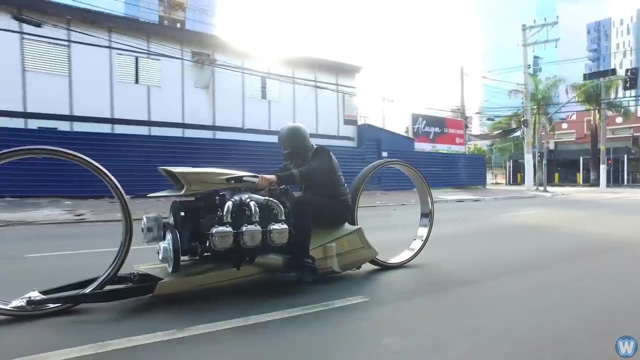 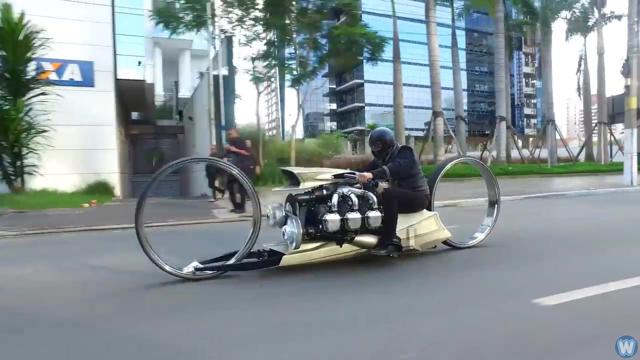 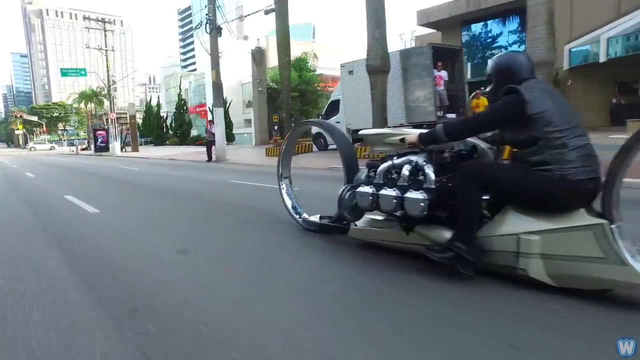 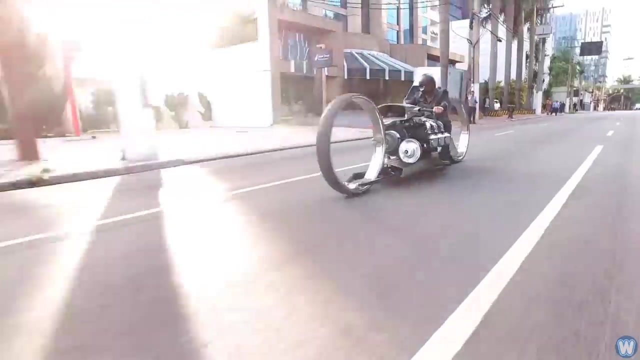 something out of a science fiction film. This ultra sleek motorcycle is powered by an actual 300 horsepower six-cylinder Rolls-Royce Continental aircraft engine from the 1960s. The engine may be a point of focus for many motorcycle enthusiasts, but the TMC Dumont also. 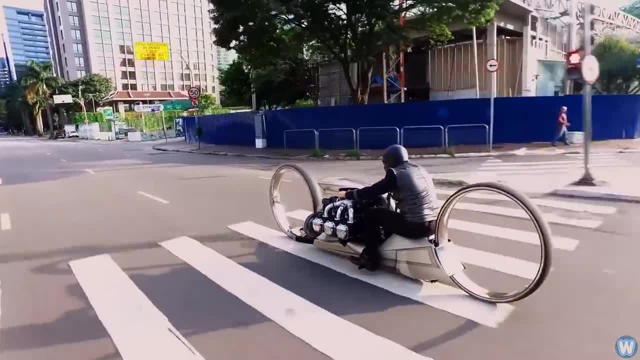 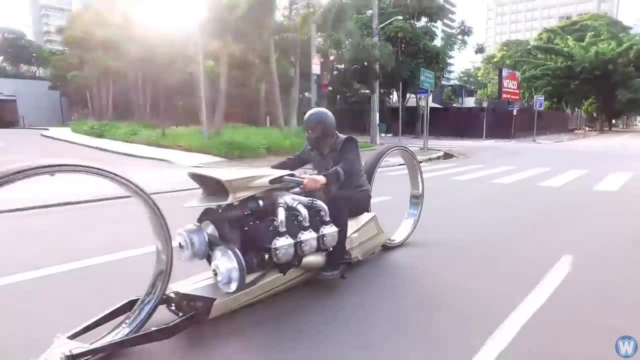 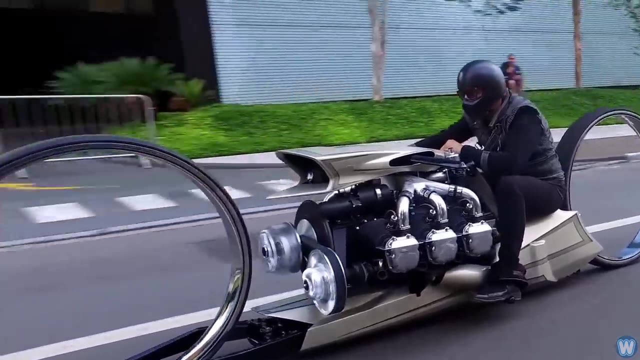 draws quite a bit of attention thanks to its unique wheels: Two massive 36-inch hubless wheels that appear to be magically attached on the bike and gives the bike an incredibly futuristic appearance. Adding to its outstanding performance is the TMC Dumont's continuous 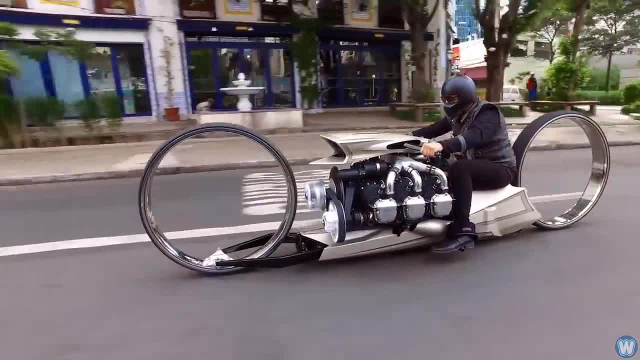 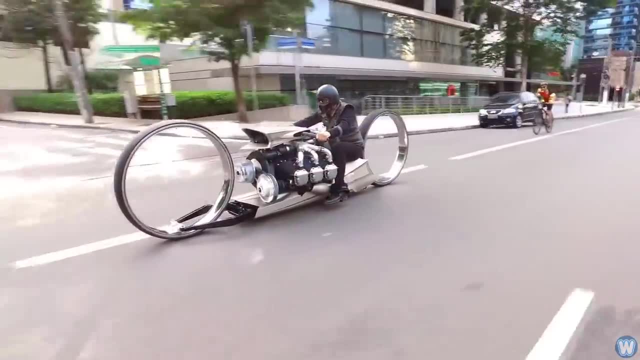 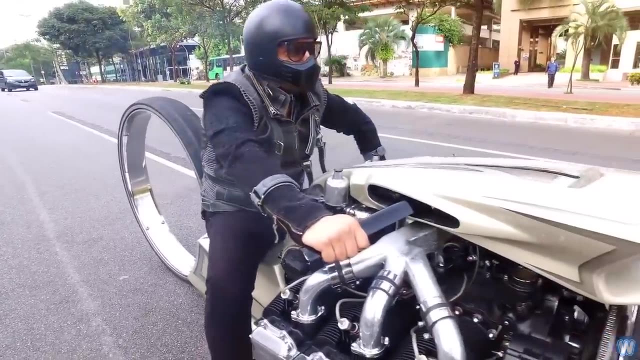 lean variable transmission, or CVT, A transmission designed, developed, created and manufactured specifically for this bike. That means this bike is an automatic, which means no clutch, no gear shifting. simply sit on the bike, start it and twist the throttle to go Sort. 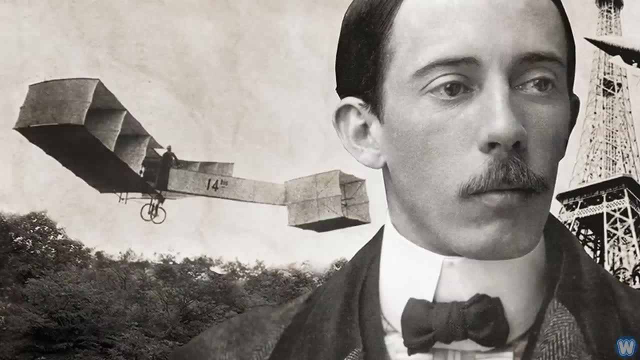 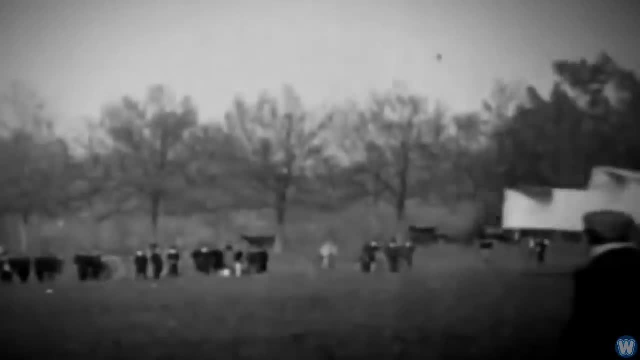 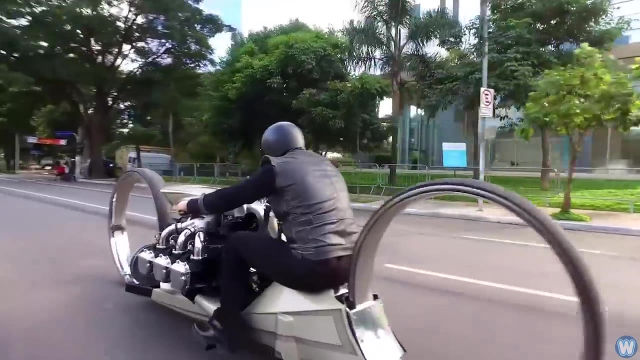 of like a scooter. The name Dumont is a tribute to Alberto Santos Dumont, who was a national hero in Brazil. It's a tip of the hat to the Brazilian aviation pioneer who, Brazilians believe, got an airplane aloft before America's Wright Brothers. 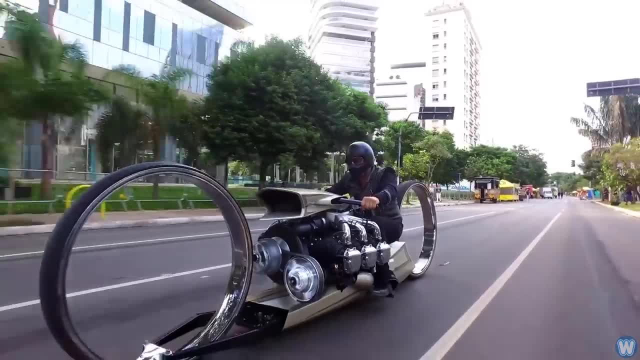 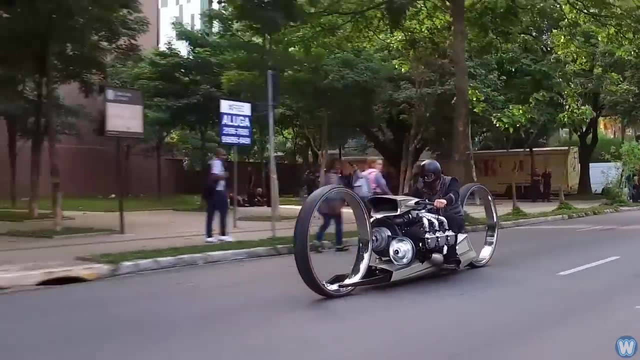 It's kind of hard to wrap your head around how the bike rides and turns, but it appears to have pivot points on the front wheel mount Which I assume makes it turn. but in the only video on Tarzo's YouTube channel showing him riding it, he only rides it in a straight. 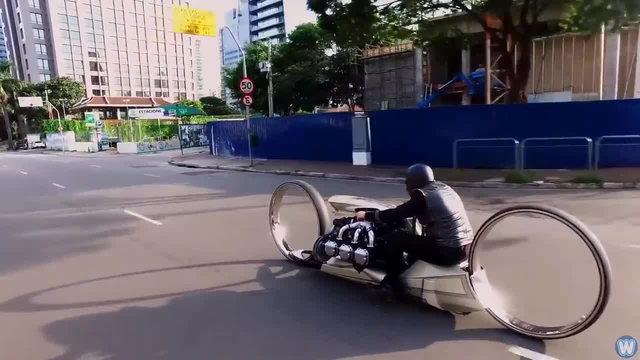 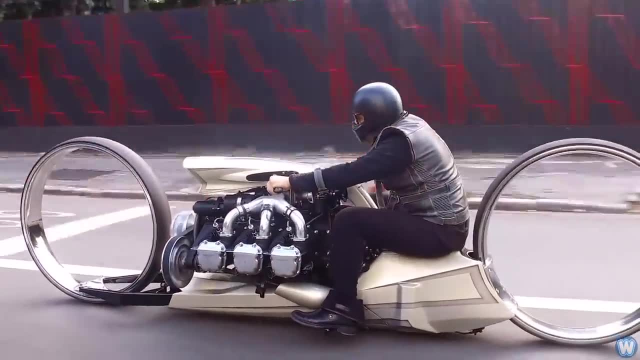 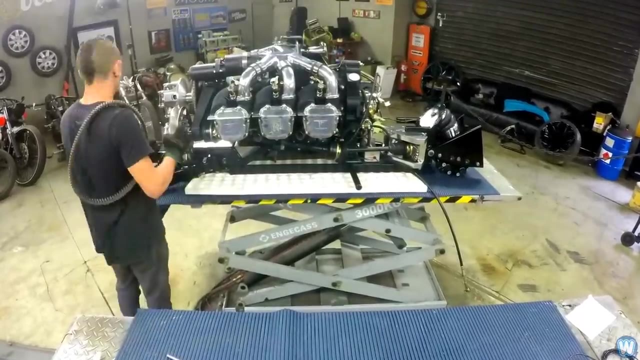 line Plus. if you look closely at the seating position, you would not want to move around too much, as you seem to be sitting an inch from the back of the bike. There are a lot of custom art bikes that are purely for show and are not rideable, but 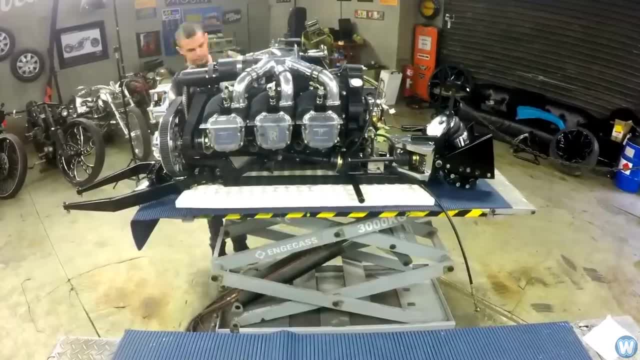 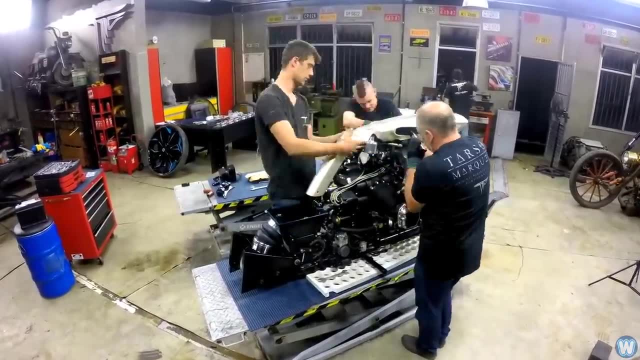 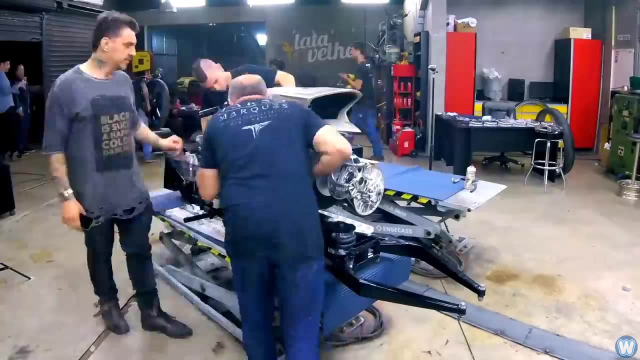 the TMC Dumont is rideable. Tarzo always rides it to bike shows instead of loading it on the back of a truck. The TMC Dumont made its debut at the Daytona Bike Week in 2018, the most important customization event in the world- and won best in show out.